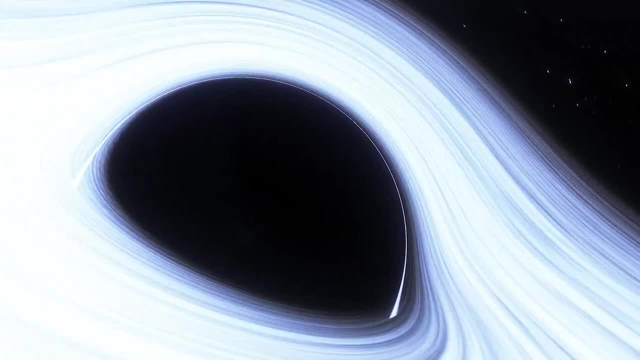 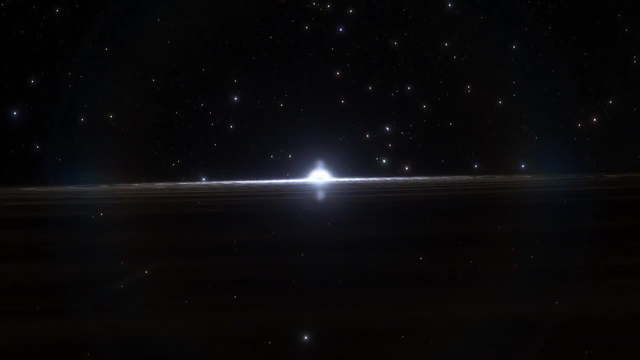 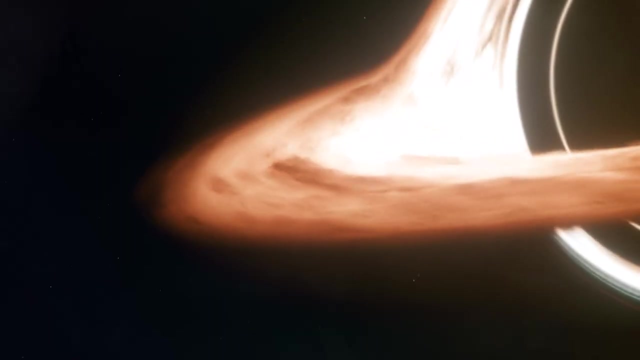 simply fall inward into the black hole in a straight line, An accretion disk forms. The flow tends to flatten into a disk in directions perpendicular to the black hole's rotation axis. because the rotation prevents the inflow of matter, Matter contracts toward a plane in directions parallel to the rotation axis until the heat. 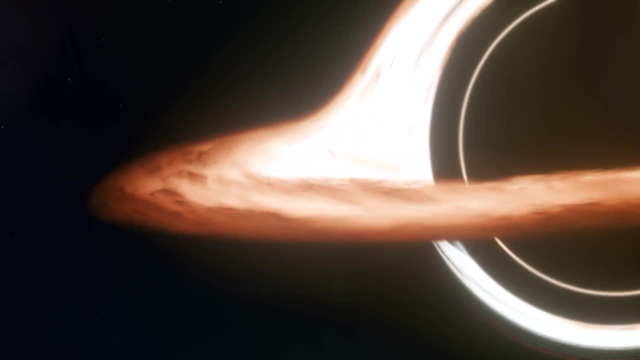 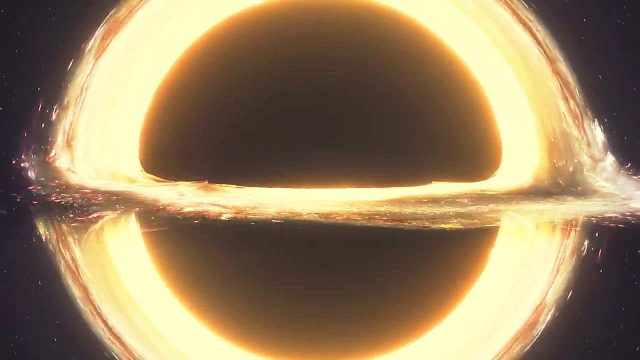 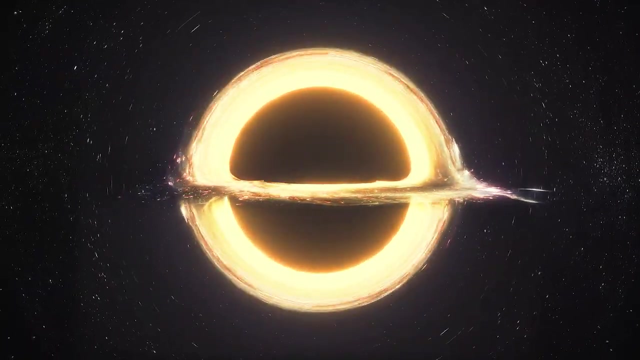 pressure inside the accretion disk approximately equals the gravitational force. The accretion disk will be geometrically thin and its thickness will be much smaller than its radial extent if the heat pressure which resists compression is minimal compared to gravity in rotation. 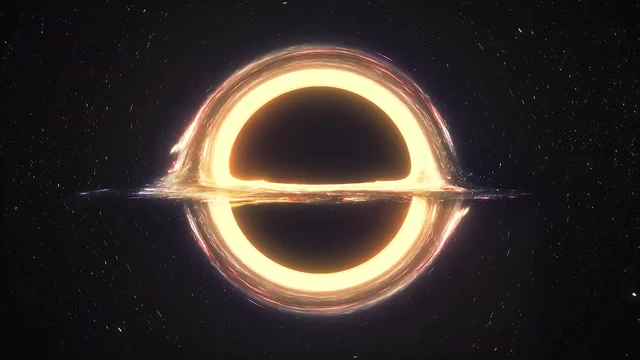 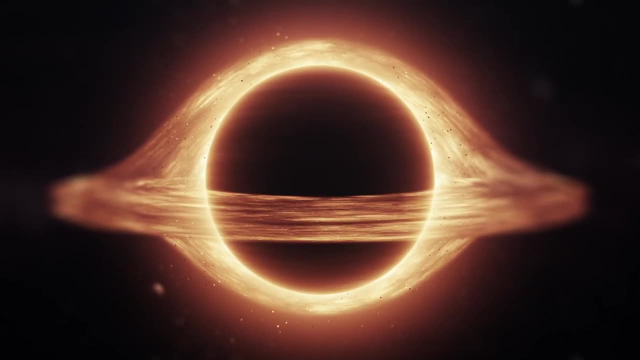 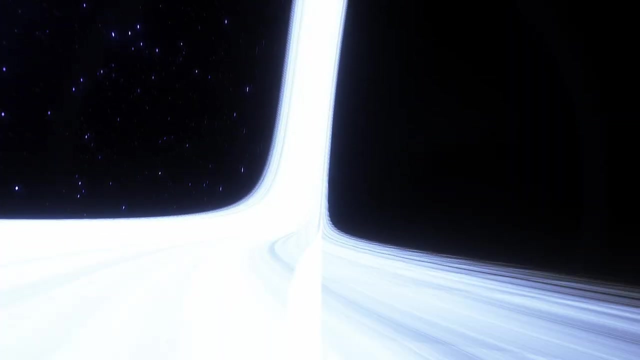 Which causes the accretion disk to contract vertically. If pressure forces are comparable to rotation and gravity, the accretion disk will be geometrically thick, looking more like a torus than a disk. Due to turbulence and viscosity, the matter within the accretion disk spirals inward. 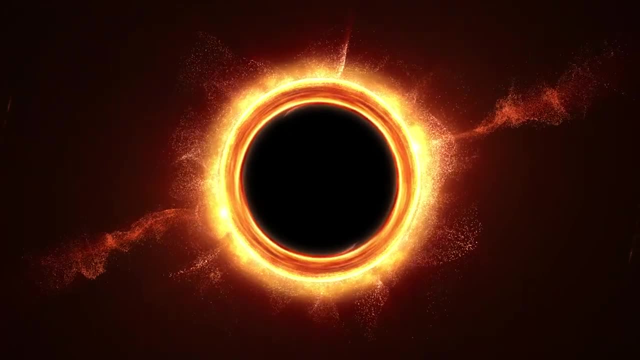 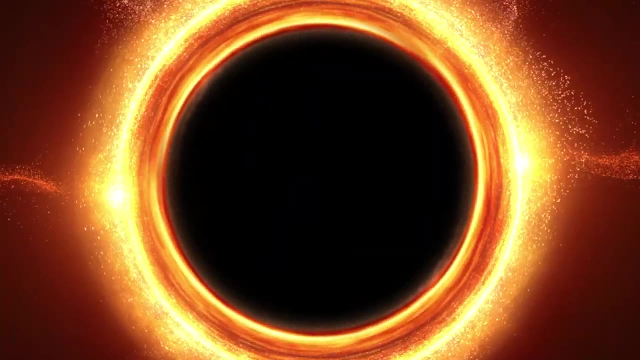 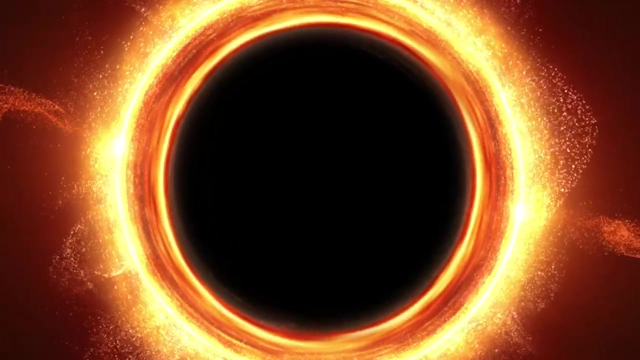 losing energy and angular momentum, The material orbiting the black hole would swiftly sink toward the equatorial plane of the accretion disk In the absence of any viscosity, turbulence or other types of friction, and then continue to travel in circular orbits. 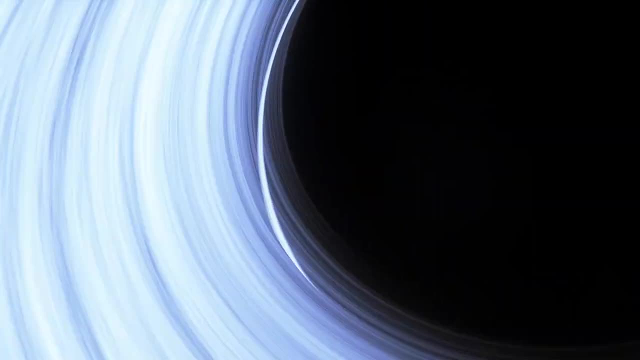 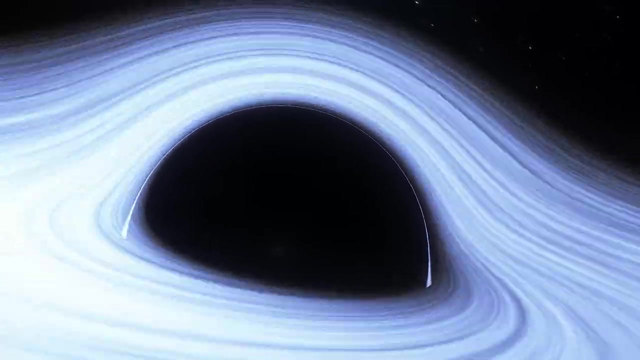 For matter to flow inward, for accretion to occur, some type of friction that dissipates angular momentum is required. Viscosity in the black hole is too low to generate inward drift at the densities and temperatures found in accretion disks. 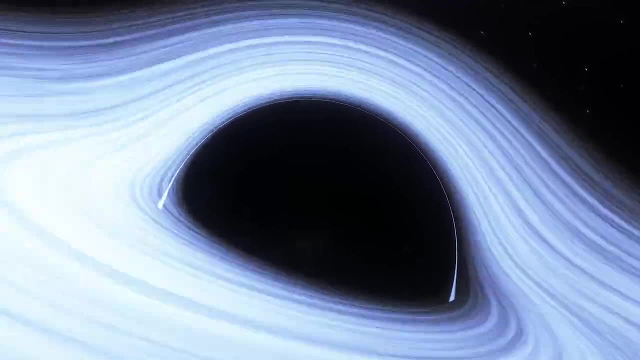 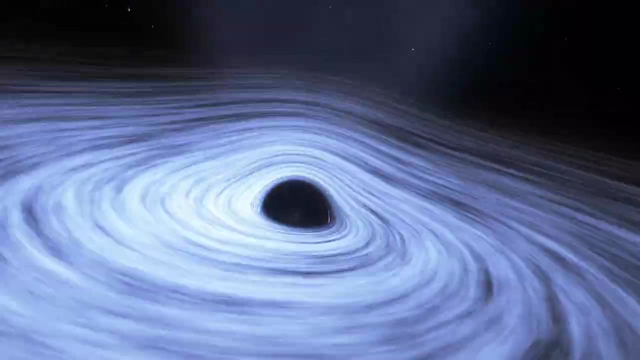 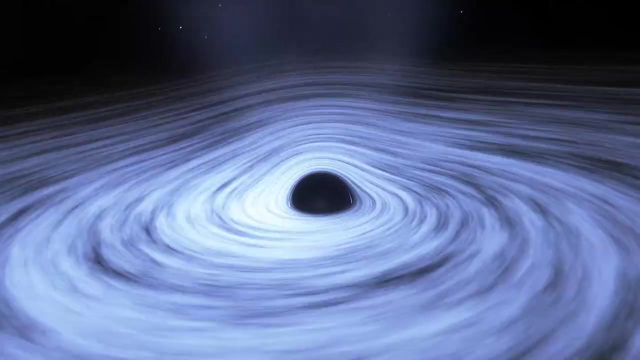 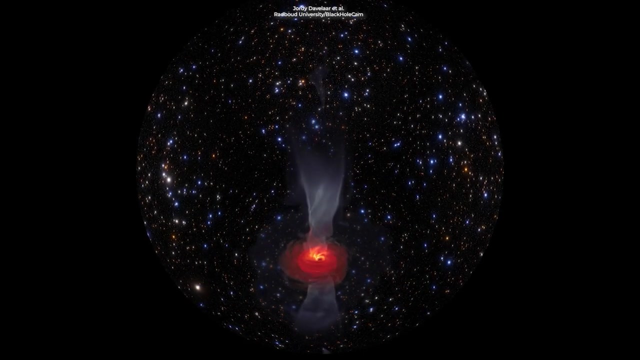 The friction is considered to be caused by turbulence due to the rotation of the black hole's accretion disk increasing any magnetic fields that already exist. The effect of viscosity that pulls matter inward while conveying extra angular momentum outward is provided by turbulence As the accreted material falls or spirals inward. accretion disks generate enormous 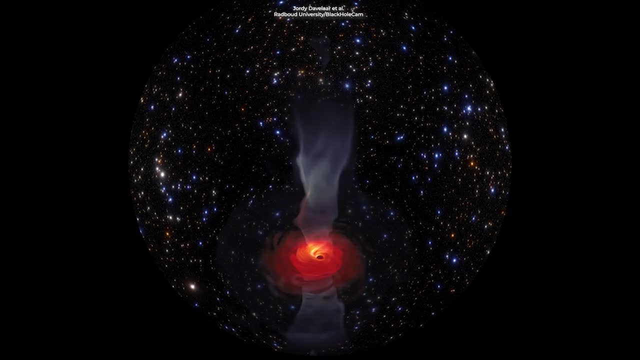 amounts of energy from converting gravitational potential energy into radiation In the black hole. accretion can release energy from the black hole In the black hole. accretion can release energy from the black hole In the black hole. accretion can release energy from the black hole.